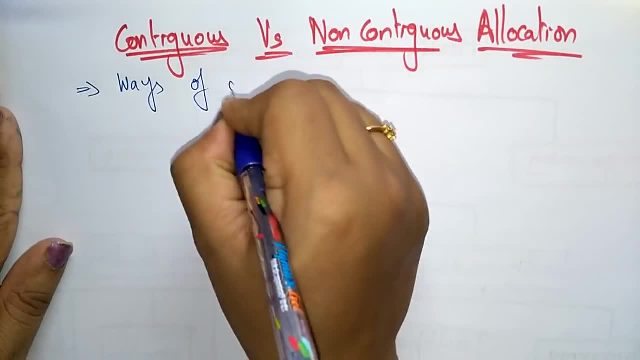 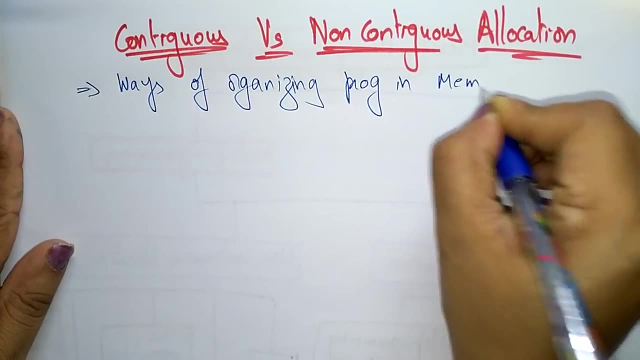 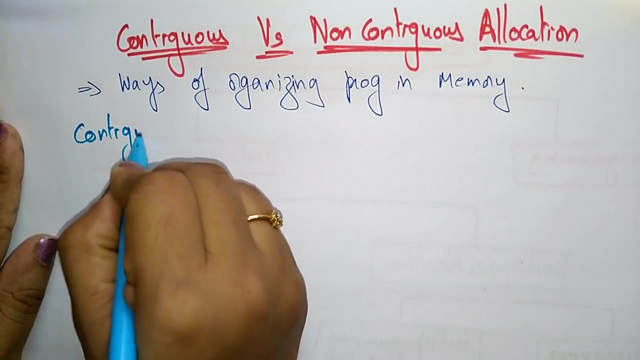 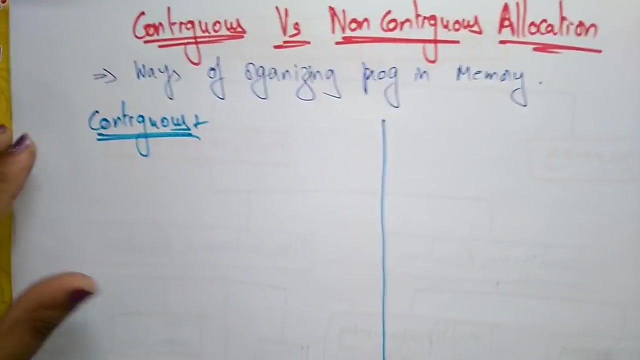 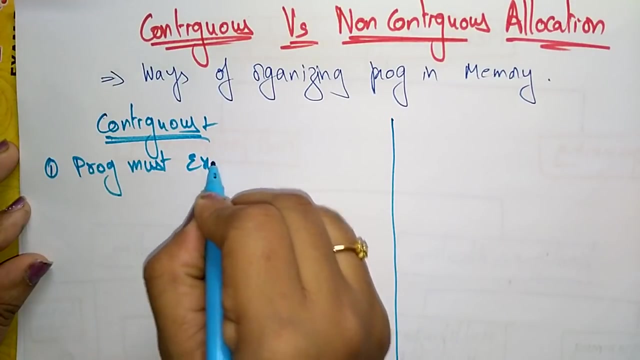 It is a way of organizing program in just. it is a way of organizing program in memory. Now let us take the contiguous. So what is the contiguous allocation? Let me take the contiguous allocation. Here, the program must be, the program must exist as a 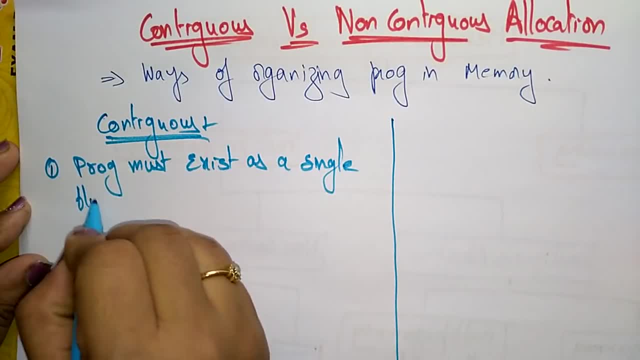 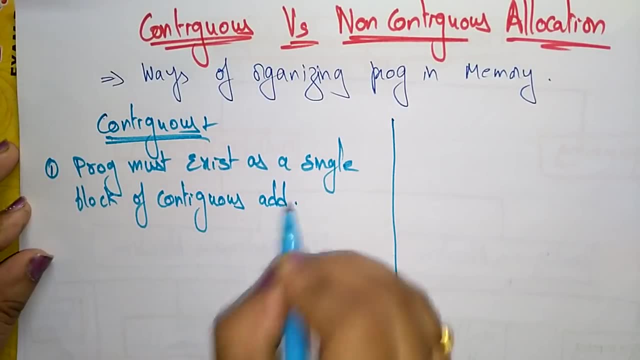 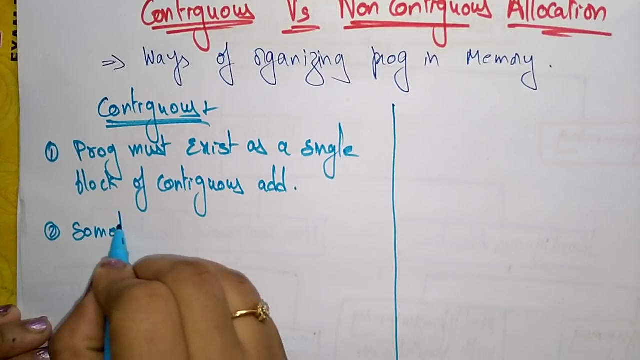 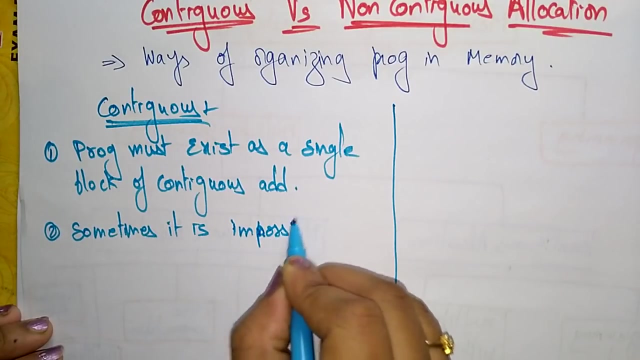 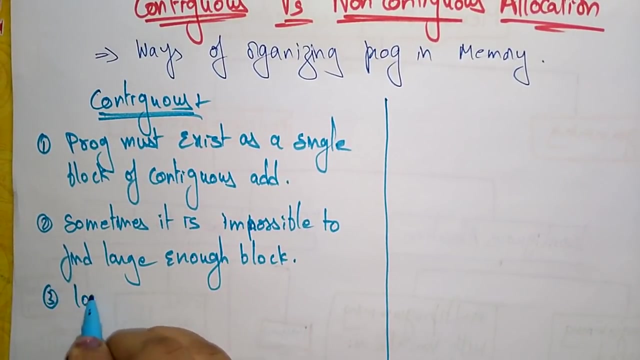 In a single block of contiguous address. So the first thing is the program must exist in a single block of contiguous address And sometimes it is impossible to find large enough block. Sometimes it is impossible to find large enough block And it is having low overhead on operating system. 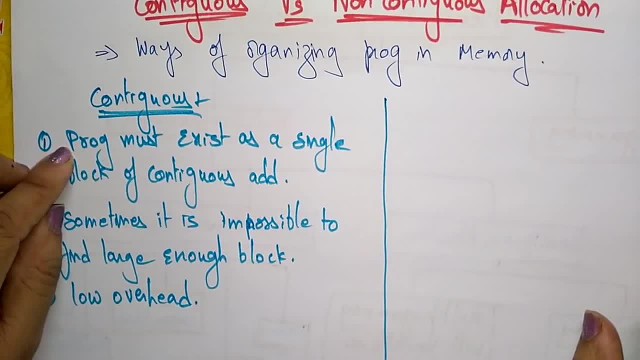 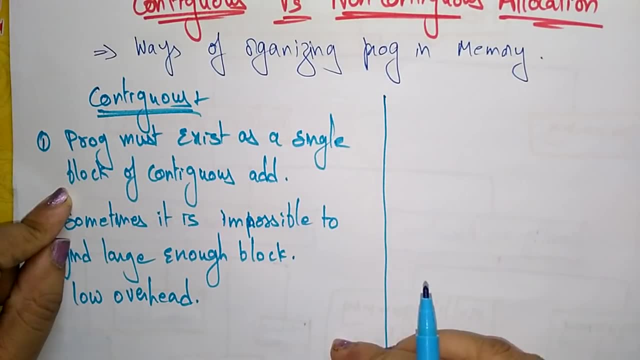 So this is about contiguous In the contiguous, The programs. the process must exist in a single block of contiguous address. So only present in a single block, with having contiguous address Means the sequence of address. Sometimes it is impossible to find large enough block. 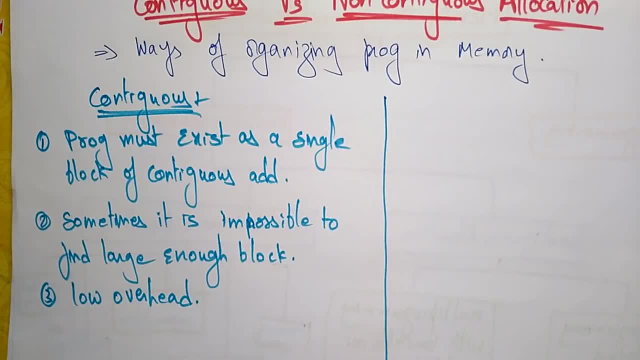 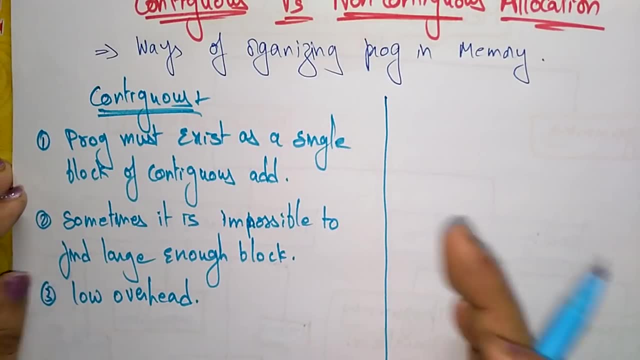 Suppose, if you get, If you want to store the data, which, If you want to execute the data or the process, that is having the large memory Means that program is having the large memory. So it is impossible to find large enough block in contiguous memory allocation. 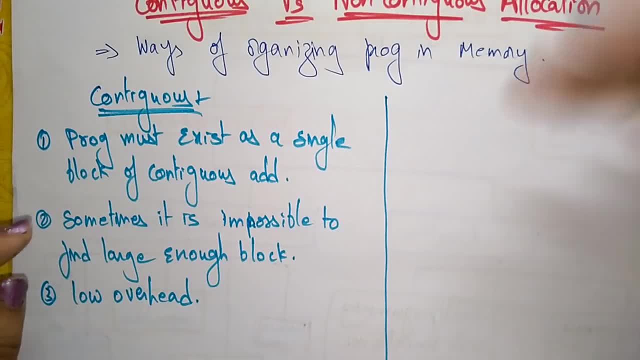 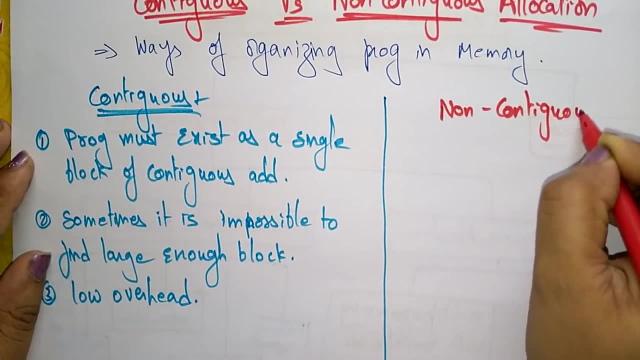 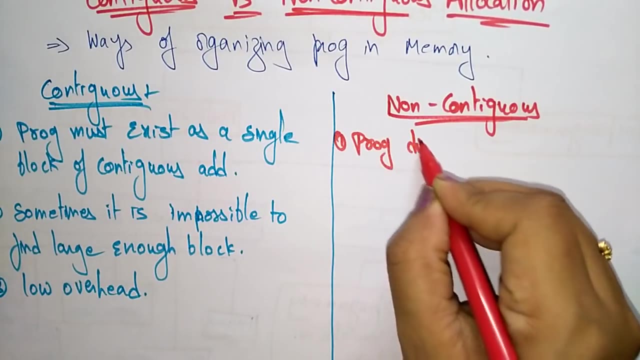 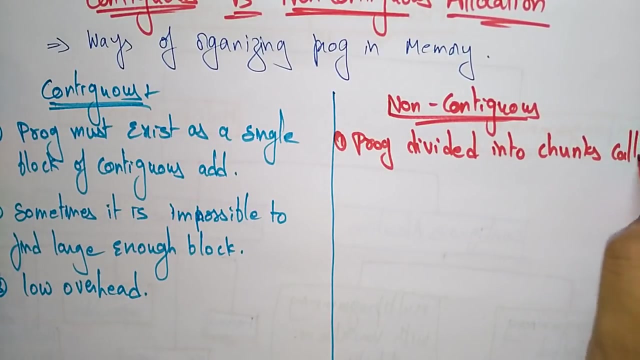 And there is a There is a low overhead problem will be there in contiguous. Now coming to the non-contiguous allocation. So what is about the non-contiguous allocation? So here the programs divided into The programs, divided into chunks, Called segments. 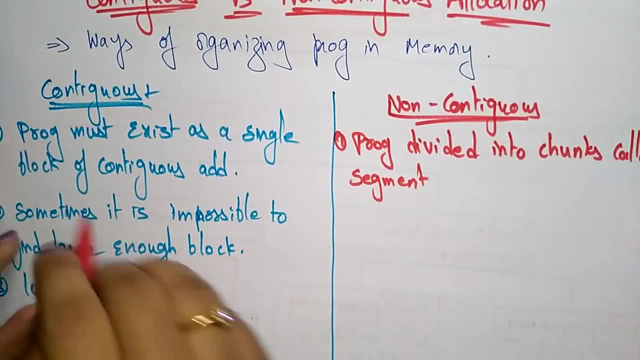 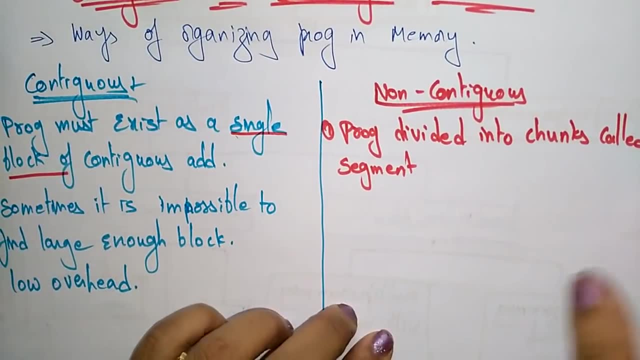 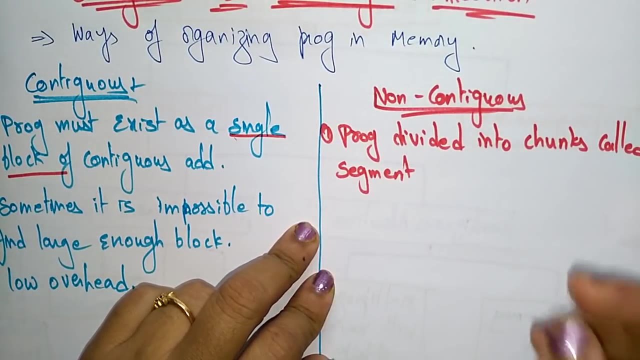 In contiguous allocation actually the complete program block Will be stored in a single block, Means the program complete program is stored in a single block, Whereas in non-contiguous allocation Program is divided into chunks called segments. The complete program is divided into small partitions.